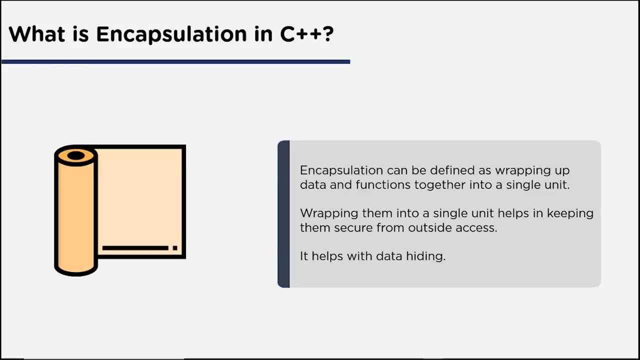 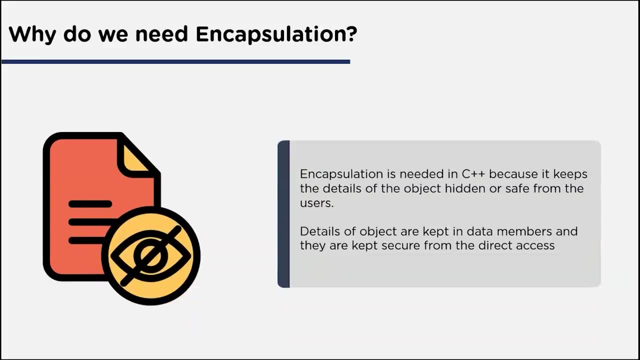 access. For example, inside a class, the variables and functions are declared and then bind together with the help of class, which also implements encapsulation. Next is: why do we need encapsulation? Hiding the details or attributes is also an important thing that one should focus on. 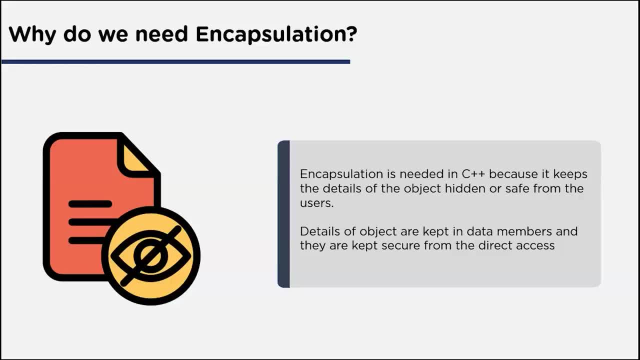 Encapsulation helps with that part. It keeps the details of the object hidden or safe from the users by securing them from the outside access. There are many implementation details that the users are not supposed to see, So these details, like the details of 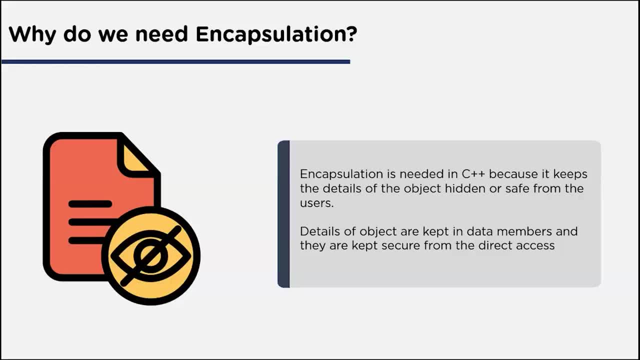 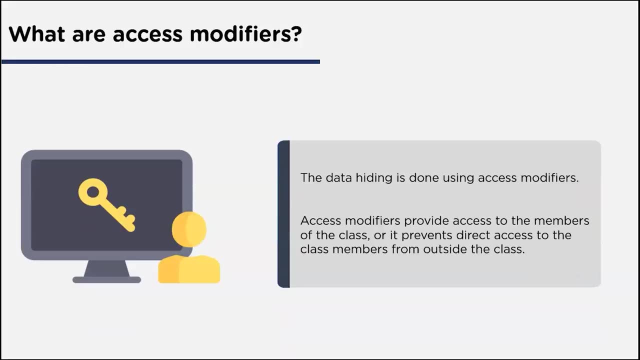 the object are kept secure from the direct access from outside the class with the help of encapsulation. The data hiding is done with the help of access modifiers. So let's Let's understand these access modifiers. The access modifiers helps in data hiding part. 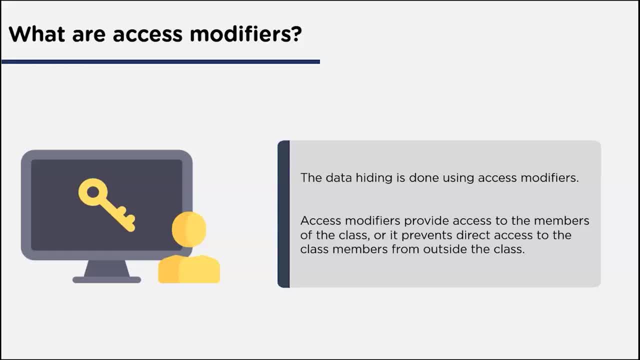 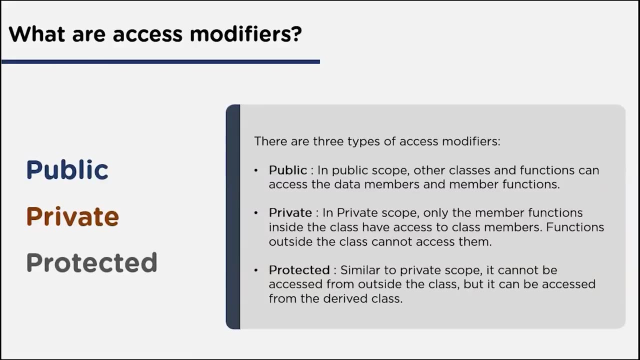 The access modifiers provides or grant the access to the members of the class or it prevents them from the direct access to the class members from outside the class. So there are generally three types of access modifiers, that is, public, private and protected. So let's understand them. 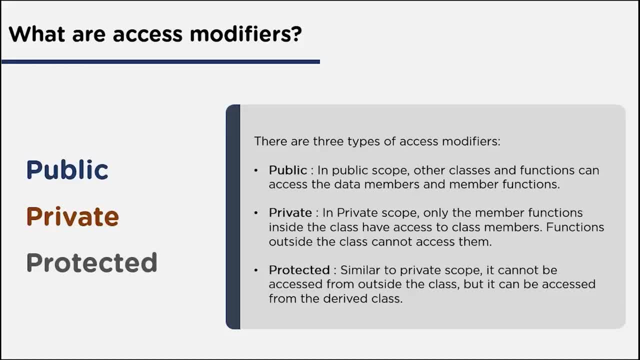 In public access modifier. other classes and function can access the data members and member functions of the public class. For example, park is a public property. Anybody can go to the park or access the park because it's a public. Nobody has to take the allowance of anybody to go to the park. 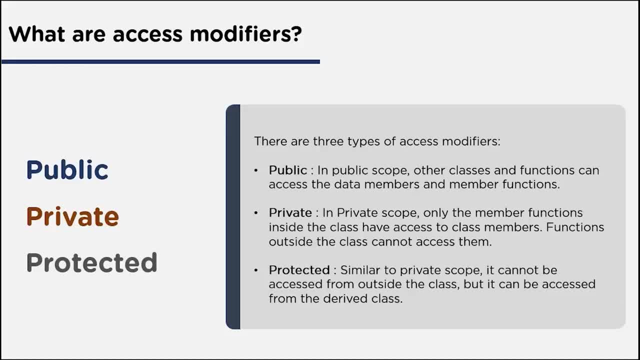 Now coming to the private. In private access modifiers, only the member functions inside the class have the access to the class. members Functions outside the class cannot access them. For example, a house is a private property. Any member outside the family cannot access the house without permission. 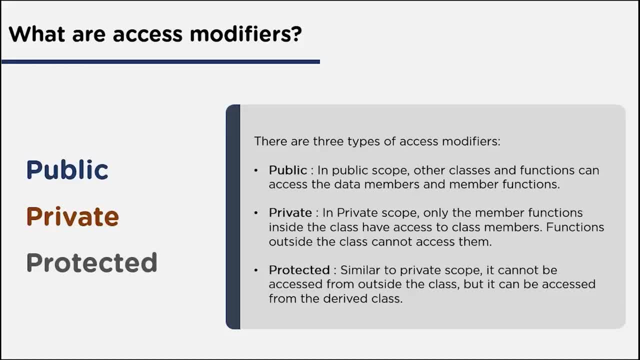 Only members inside the family can access it because it's a private property. Now let's understand protected In protected access modifier, similar to private scope. it cannot be accessed from the outside class, But it can be accessed from the derived class. The derived class is also called the child class. 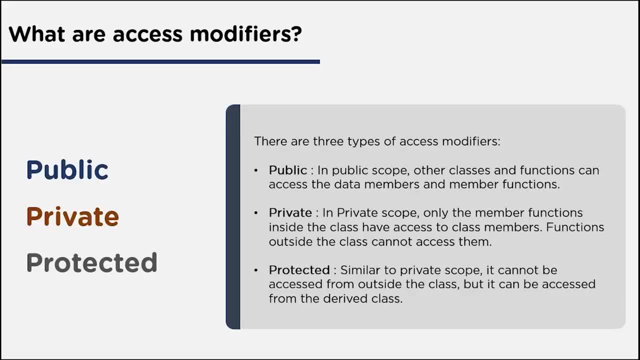 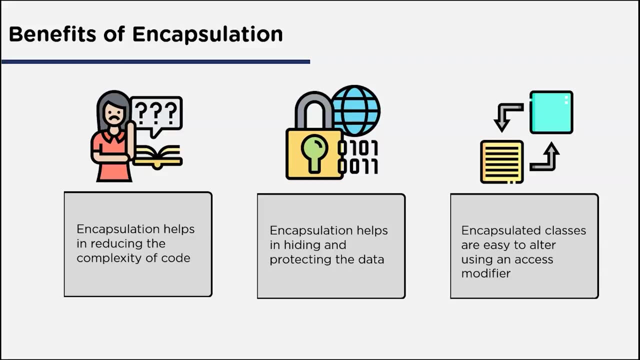 Also, the protected member of a class can be accessed from the friend function. So as we have understood about these access modifiers, now let's understand the benefits of encapsulation. Encapsulation helps in reducing the complexity of code by hiding the irrelevant data or information. 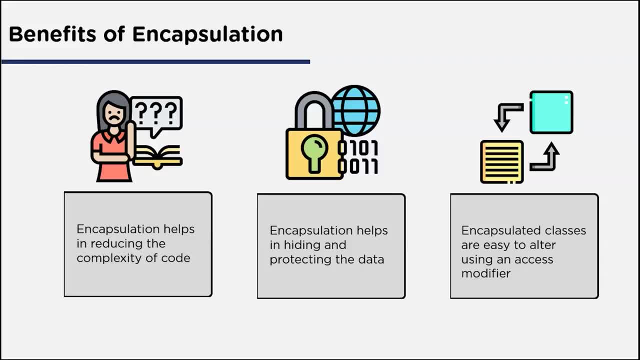 And by doing so It reduces the complexity. Second is: encapsulation helps in hiding and protecting the data by wrapping the data and function together, which are generally complex, and by doing so provides a simpler view to the user. With the help of encapsulation, the variables of the class can be hidden from other classes. 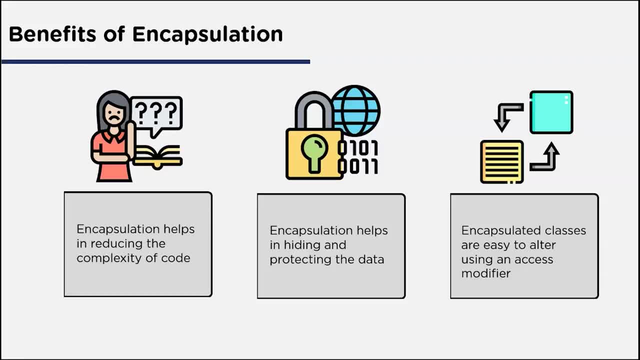 Third is encapsulated classes can easily be altered using the access modifiers. That is To change the entire program. all we need to do is to change the access scope of the variables. that can be private, protected or public. So these were some benefits of encapsulation. 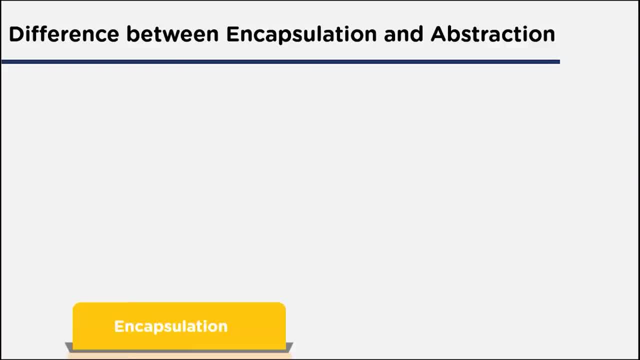 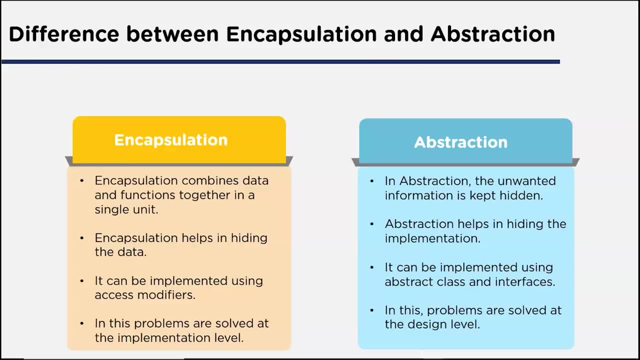 Now let's go ahead and understand the difference between encapsulation and abstraction. Both of these concepts are similar in some ways, But now we will discuss their differences. So let's start with encapsulation- Encapsulation- Encapsulation- Encapsulation is a function of the data and functions together in a single unit. 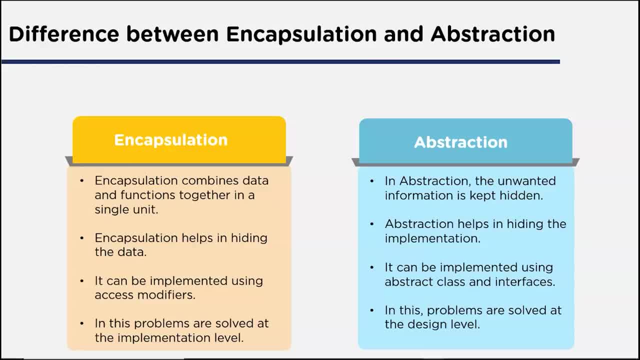 Whereas in abstraction the unwanted information is kept hidden. Encapsulation helps in hiding the data and helps in providing an easier view. Abstraction helps in hiding the implementation details. Encapsulation can be implemented using an access modifiers, Whereas abstraction can be implemented using abstract class and interfaces. 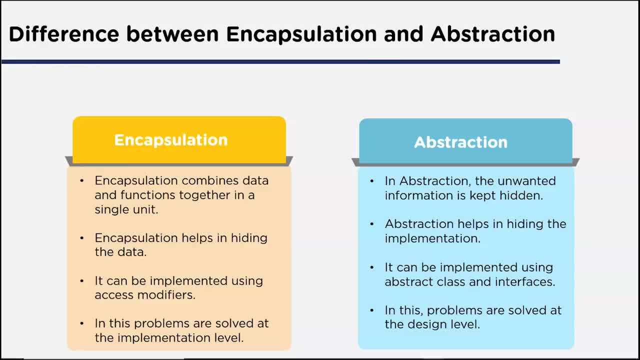 In encapsulation, Encapsulation, Encapsulation, Encapsulation, Accapation, Encapsulation, Accapation, Encapsulation, Accapation, Accapation. In encapsulation Problems are solved at implementation level and in abstraction problems are solved at 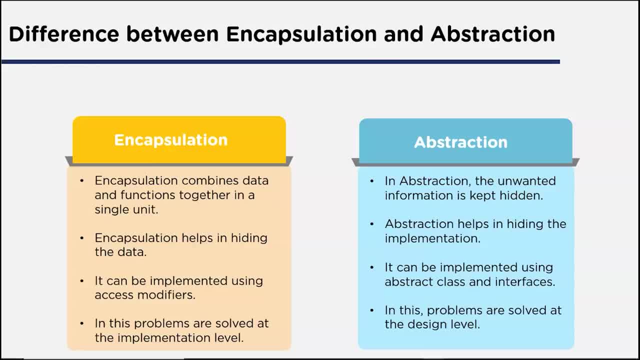 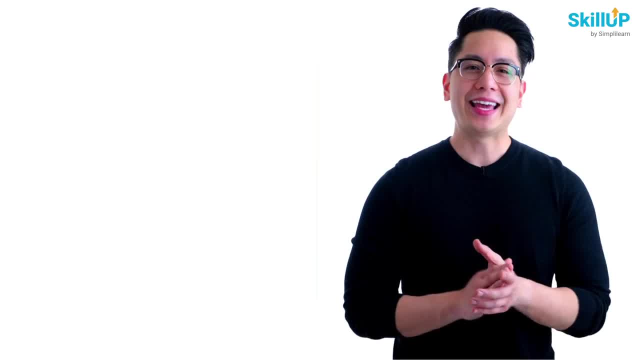 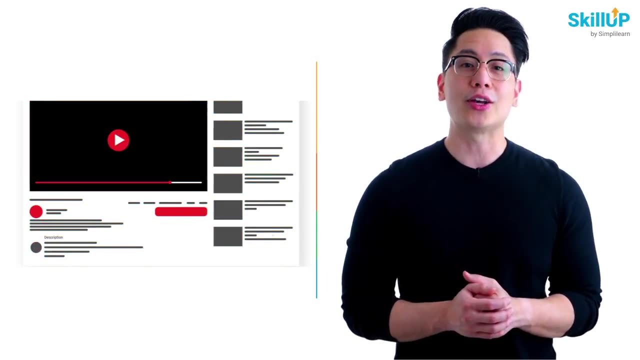 design level. So these were some differences between encapsulation and abstraction. Let's go ahead and do some practical examples on this topic. If getting your learning started is half the battle, what if you could do that for free? Visit: scale up by simply learn. 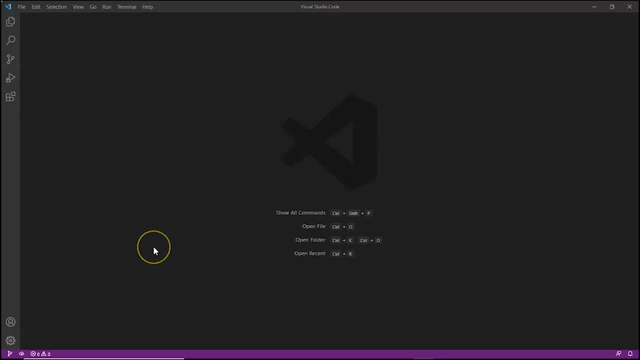 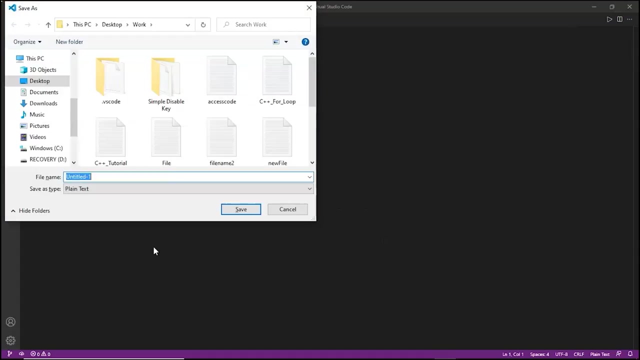 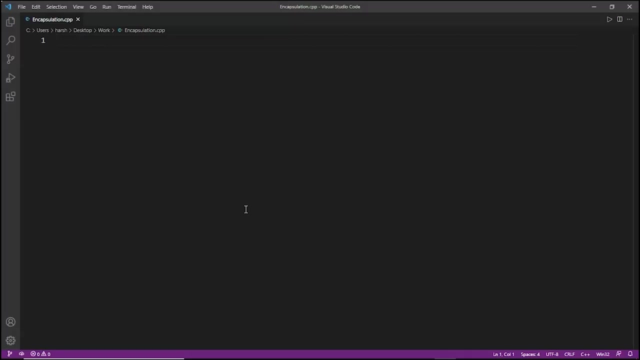 Click on the link in the description to know more. so this is our code editor, that is, Visual Studio code. and now let's create a new file and let's name it encapsulation dot CPP. so first of all, we know, in encapsulation we can make variables inaccessible by making their scope as 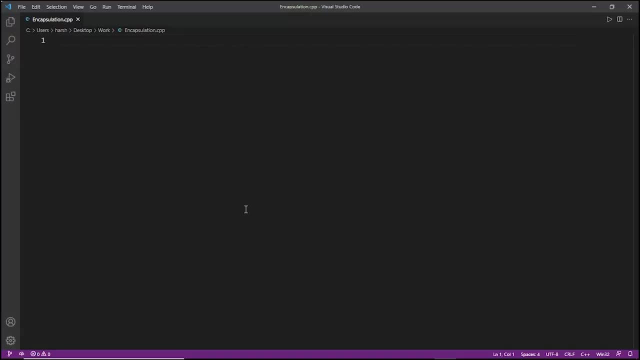 private. so in this example we will do that. we'll make the salary of an employee as private and then, using the setter and getter methods, we will set the value of salary and return it as well. the setter- getter methods are generally used in these kind of situations, where the variable we want to 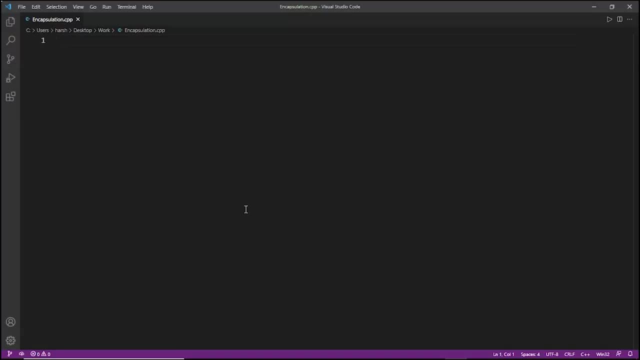 access is private. so now let's start. first of all, we will create the main function, but before that let's add the header files, now using namespace standard. now we'll start with the main function and inside the main function. first of all, we will create an object by declaring the class. 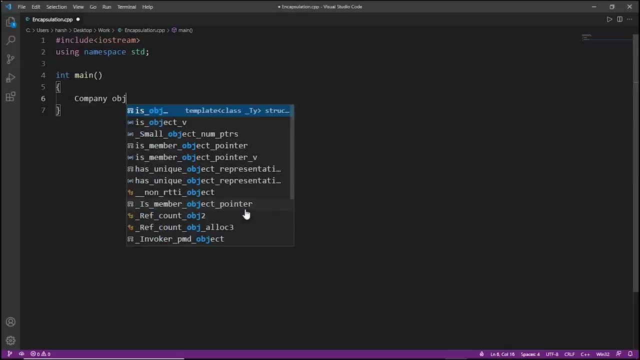 name. let's say the class name is company, the object name is OBJ. now, using this object, we will call the set function, or we can say the setter function. we will name it as set salary. let's say, and we will pass two values, thirty thousand and six thousand. 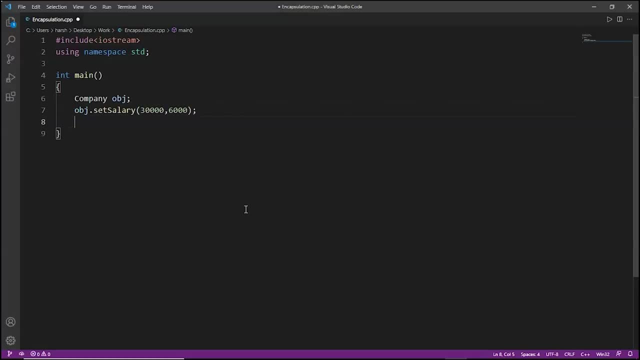 one would be the full-time salary and one would be the overtime. all right now. after that we can display those and we can write total salary, and after that we can call the get function to return the salary. as the getter function is used to return the output and set function is used to it set the. 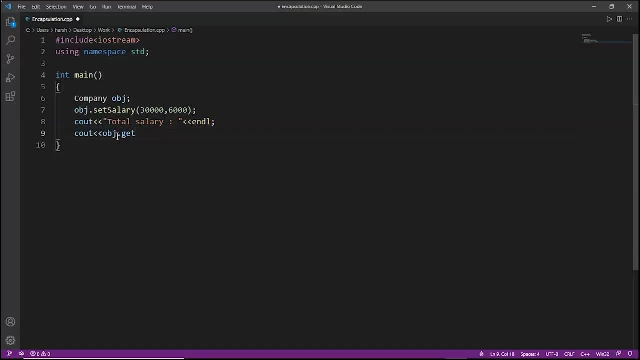 values. so we'll write OBJ dot get salary, so the salary we will display over here, and after that we can write the return zero. now the main function is done. now let's start with company class, company class company and inside this class, first of all inside the private school. this is the 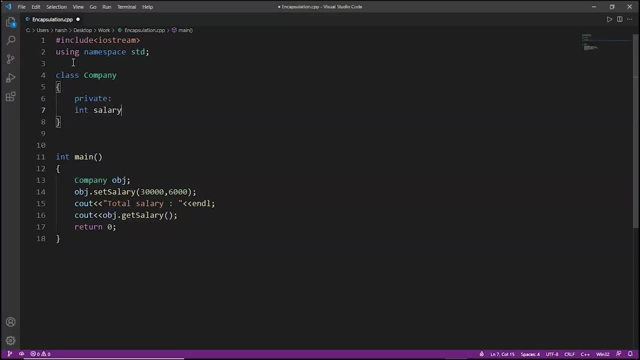 private school and this is the variable salary. now, this variable salary is private, so no member outside the class can access it. but using the setter and getter methods, we will access this variable and we will set the salary and then we will return it all. right now. public scope inside the 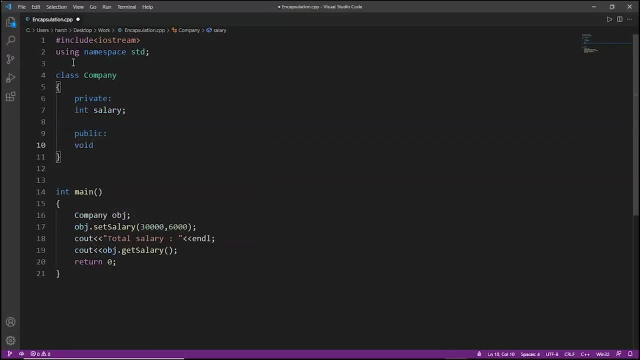 public scope. we will write the setter methods: void, set salary and in full-time and overtime. so these are two variables. this 30,000 that we are passing is a full-time salary and this 6,000 is an overtime salary, so we need to add both of these salaries in. 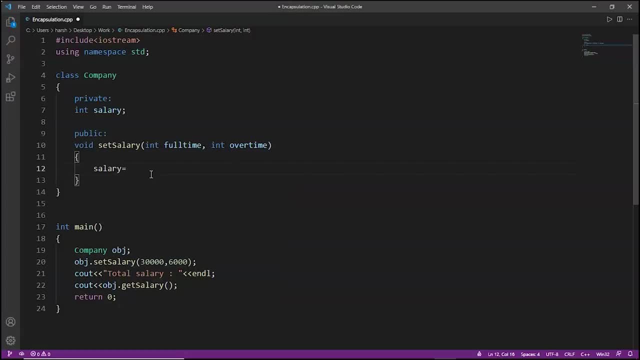 this part, so we'll write: salary equals full time plus overtime, so this would be the total salary and let's just do this. all right, so this set salary function is done. this is the setter function. now we have to return using the getter function, so we'll write the data type: int- get salary. 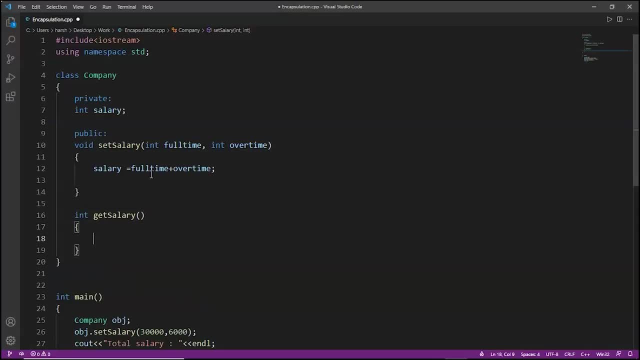 now, inside this function, we will simply return the variable salary, as we can see, and once the class, we'll use this semicolon. all right, pretty much everything is done, and now we can save it. and let's try. as you can see, total salary is thirty six thousand as thirty thousand plus six thousand, so it is. 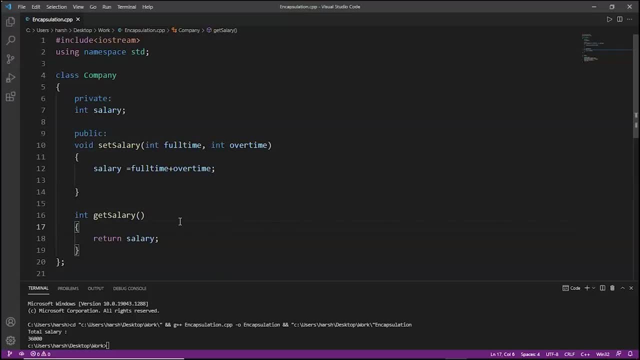 working fine. So this is how we can access these private variables using these setter and getter methods. Now let's do another example. This example of encapsulation will also be pretty much the same. We'll do the setter, getter methods in this one as well, But in: 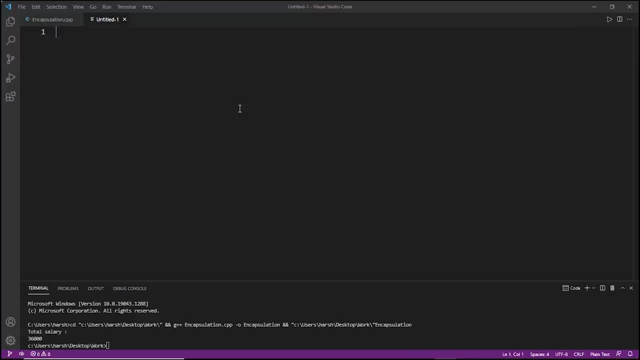 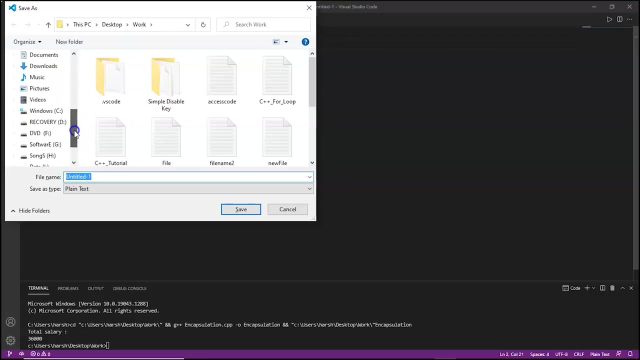 this example, we'll find the area of circle. Alright, let's start then. first of all, we'll include the header files, that is, hash, include IO stream and the namespace standard. We also forgot to save this. Let's name this one as, first of all, the location is work. Now let's 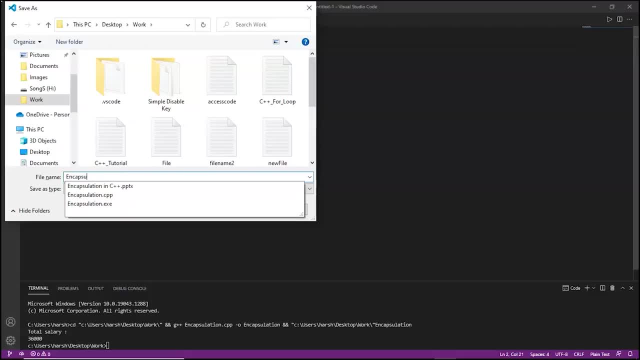 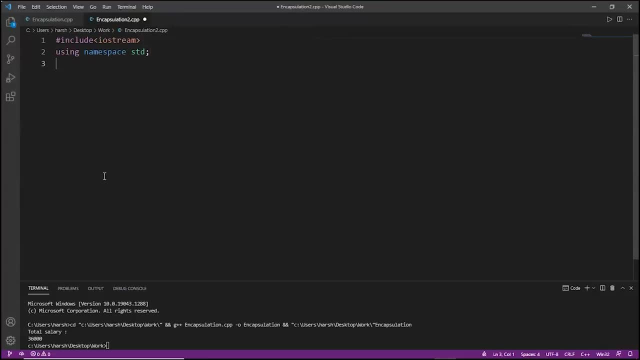 name it as encapsulation two dot CPP. Alright, now the header files that I did. now we'll start with the main function first of all. Now, inside this main function, we'll create an object. first of all, we'll write the name of the class. that is ball Now. the name of the object is OBJ. Now, using this, 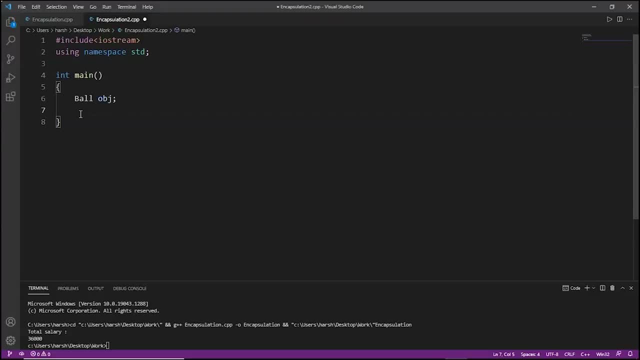 OBJ object. we will call the setter function. that is the set area function, and we will pass the radius. Alright, OBJ dot set area. This is the setter function. Now we will pass the radius. Now. now we can display the area by calling that getter function, But before that we will display a message. 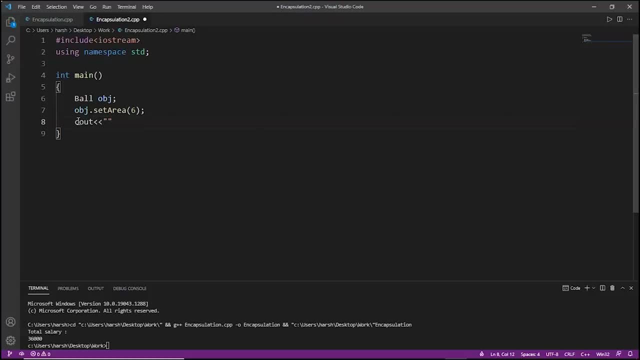 Right area of ball is get area. alright, now we will call that get a function, get area. all right, the main function is done. Now we need to create the class. 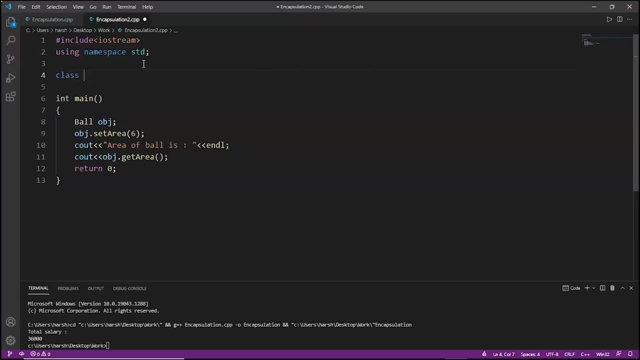 class ball inside this class private scope. inside the private scope will create that variable area and let's make its data type as float, because we know that there are chances that the answer could. 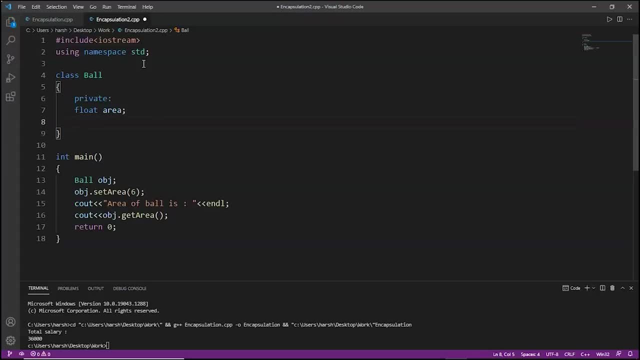 be in decimal form, because we have to use pi in that, because the area of circle is pi r square. so three point one, four is the value. so that is why we are using float as the data type. all right now, in the public scope, we'll set the radius inside this function: set area and in radius. 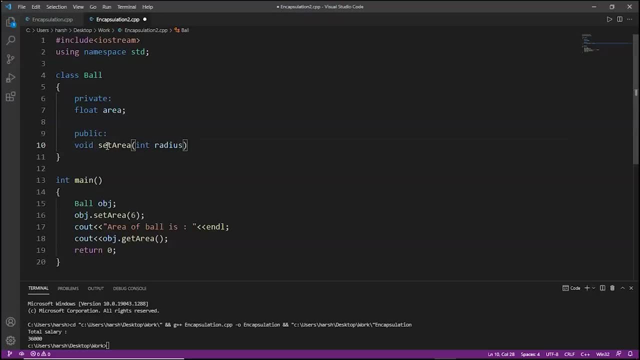 this is the radius, that is six that we are passing, this is the art, this is the parameter and inside the function area equals. we know that pi r square is the formula, so we'll write three point one, four, that is the value of pi, into radius again, into radius r square. all right, so this is the area. 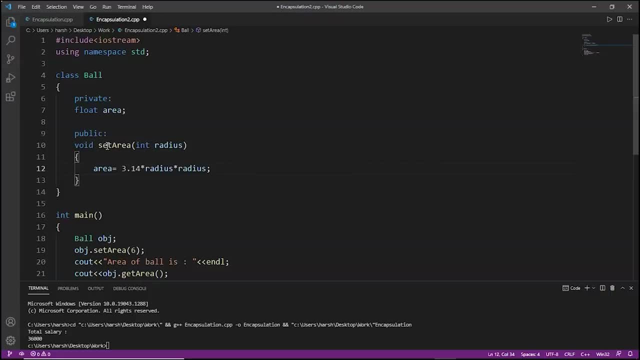 of circle or ball. we can say after that: float is the data type. now we have to return the area using the getter function, float getter. its name is get area, get area, and we'll simply return the area variable. all right, after that we can use semicolon in the end and pretty much everything is done, so let's save it. 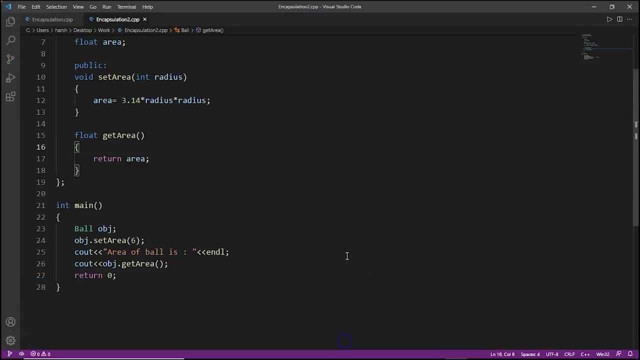 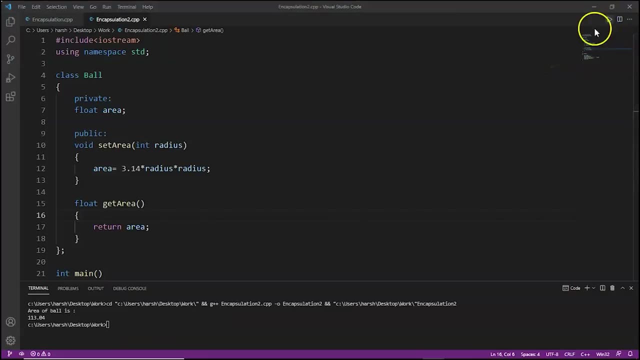 and let's check it if it is running fine or not. okay, as you can. C area of ball is 113 point zero four. so if we multiple 3.14- that is the value of pi- width 36, that is 6 into 6, it will give you 113 point zero four. so this: 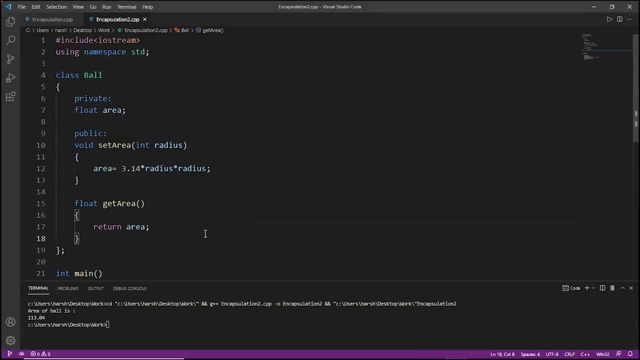 is the right answer and this is how we can find the area of ball or something like that. and, as we can see here, the area is private and using these set, area and get area methods- that is, the setter and getter methods- we are accessing this private variable that is area. so these 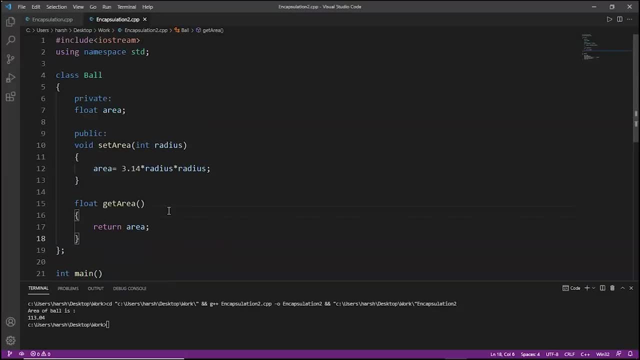 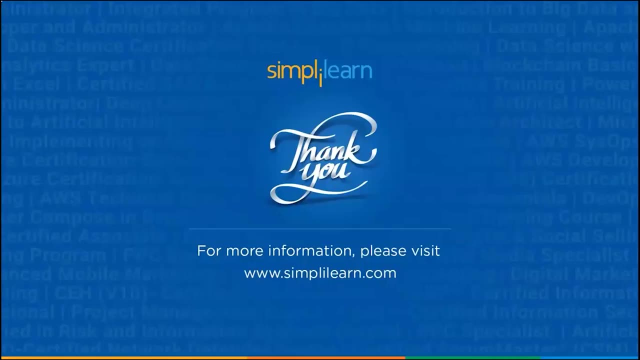 were two examples of encapsulation. you can try these examples as well. alright, guys, with that we have come to the end of this session. if you like this session, please give it a thumbs up. I hope it really help you all. thanks for watching, stay safe and keep learning hi.